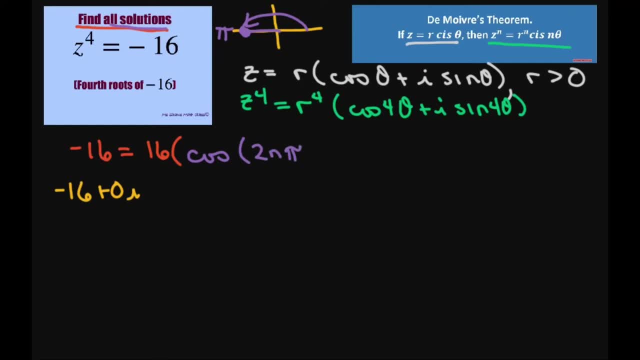 That gives me all the rotations, And then we're going to have plus our pi. Now you have to add your sine and do the same thing: n pi plus pi. This is for all solutions. n is an integer, So let's just say n is integer. 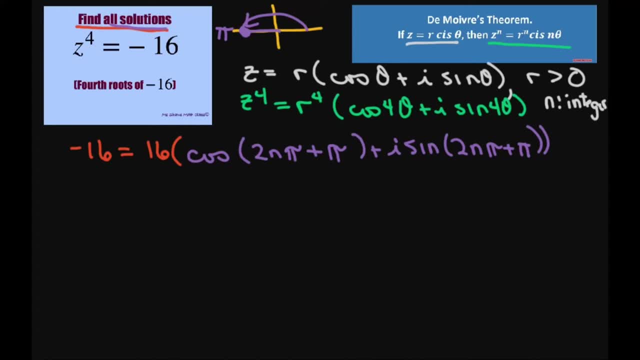 Alright, now that we have that, what we're going to do is look for our r. If this is 16 and this is r to the power of 4, our r equals 2.. And remember, it's not negative 2.. 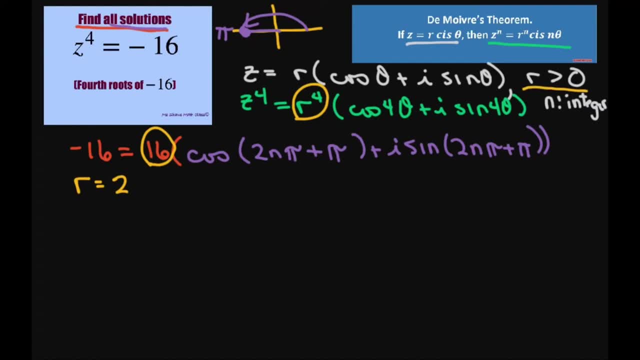 Our r has to be positive. I know that's kind of a confusing part, but r has to be positive. Alright, now what we want to do is match up these angles. 4 theta- we're going to match up to this. 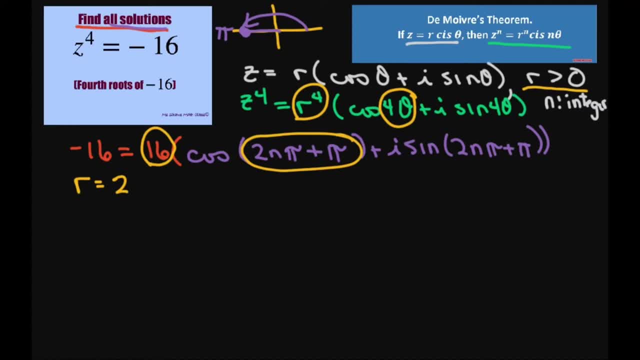 Because we're trying to get all solutions. So we're going to do 4: theta equals 2, pi n plus pi. I can just rearrange it. And when you solve for theta, you're going to get theta equals. you divide both sides by 4.. 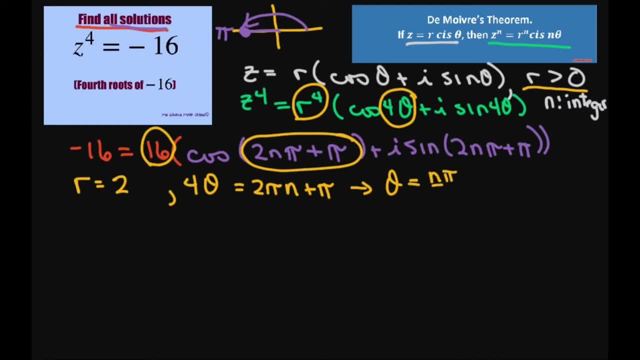 You're going to get n pi divided by 2 plus pi divided by 4.. And I can simplify this by getting my common denominator as 4 and factoring out a pi. That's going to give me 2 n plus 1 times pi. 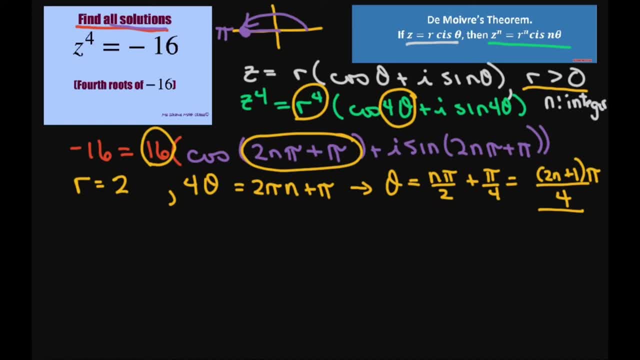 Now that we have that, let's write our new equation as: z equals 2, that's your r times cos of your angle. Now your new angle is 2 n plus 1 times pi divided by 4.. Alright, and then do the same thing. 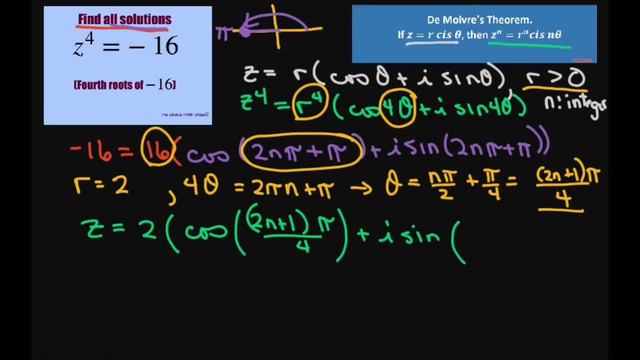 Plus i times sine of 2, n plus 1 times pi divided by 4.. Alright, and this is 4. since we have 4 here, the 4th roots, Our n, is going to be 0,, 1,, 2, and 3.. 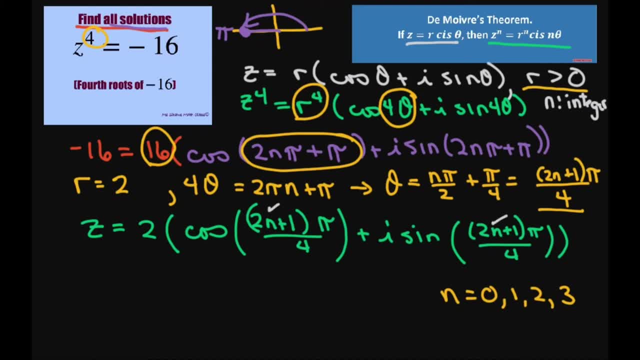 So on the next slide, what I'm going to do is substitute in 0.. You're going to get pi divided by 4's. We're going to get a lot of pi divided by 4's. So basically, you want to maybe copy this down. 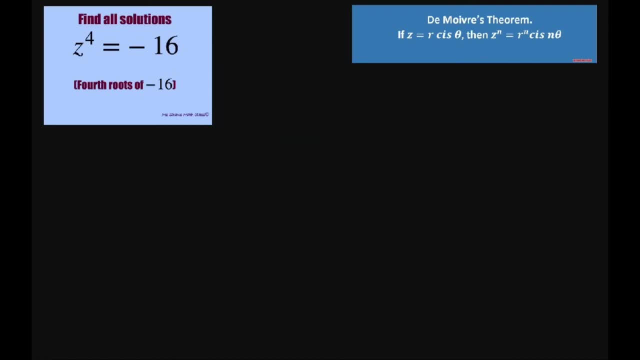 And we're going to go ahead and start with this. So we're going to get first for n equals 0.. That means we're going to have z equals 2 times square root of 2 divided by 2, plus square root of 2 divided by 2i. 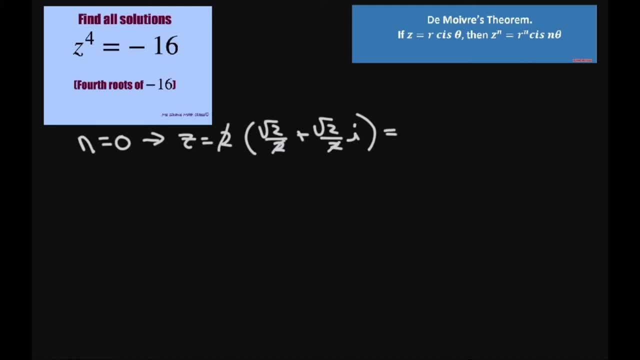 What happens is that those 2's will cancel out. So this is going to give you square root of 2 plus square root of 2 times i. Alright, now we've got to go all the way to 3.. So n equals 1.. 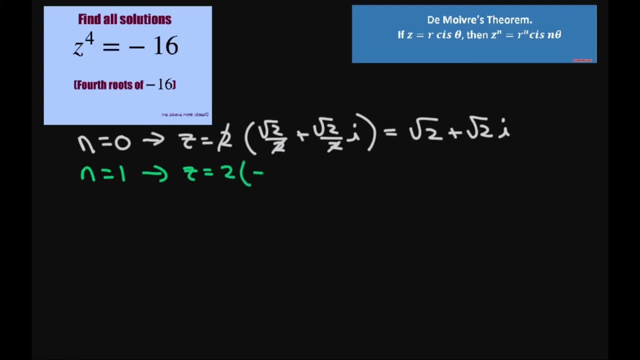 This is going to be: z equals 2 times negative square root of 2 divided by 2, plus square root of 2 divided by 2i. The 2's will cancel, so you get negative square root of 2 plus square root of 2 times i. 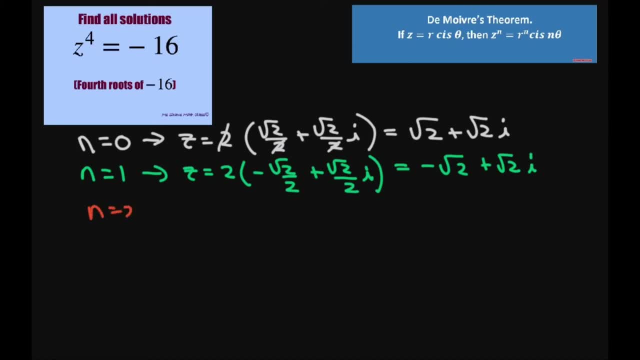 Now let's try n equals 2.. That one's going to give you z equals 2 times negative square root of 2 divided by 2i. That one's going to give you z equals 2 times negative square root of 2, minus square root of 2 divided by 2i. 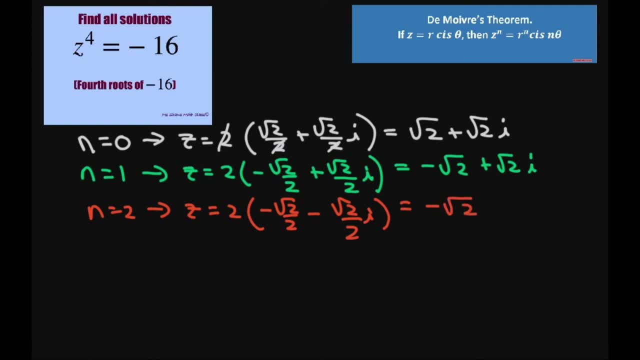 The 2's will cancel out. so we're getting this. We have 4 different solutions And finally, n equals 3.. That's going to be z equals 2 times square root of 2 divided by 2, minus square root of 2 divided by 2i. 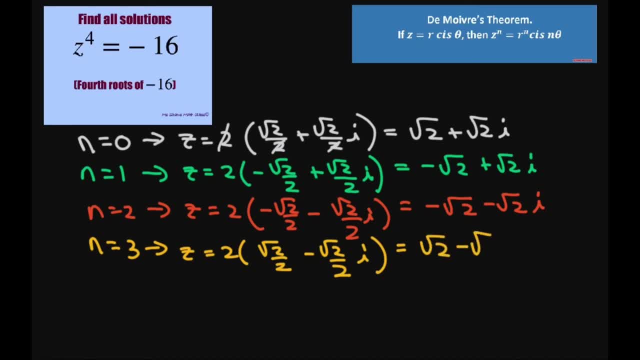 This is going to give you square root of 2 minus square root of 2. Square root of 2 minus- whoops- square root of 2i Forgot my i. All right, So your four solutions are all right here. C equals these four solutions here.